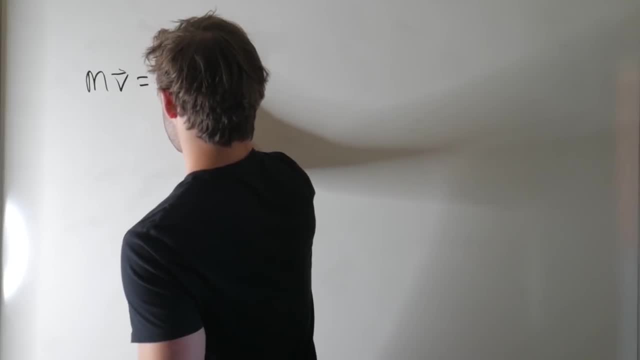 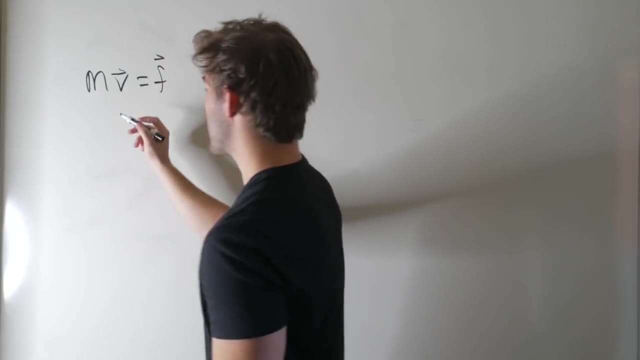 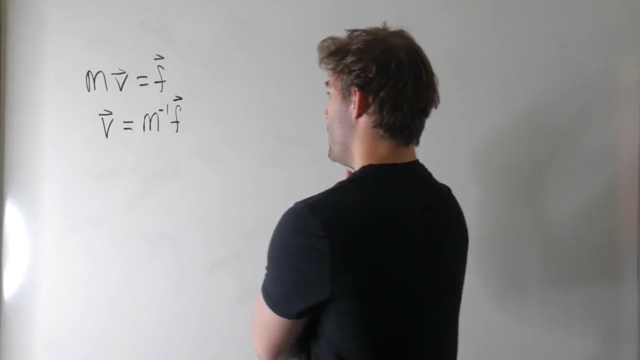 times some vector V, giving us some other vector F. Well, since M is invertible, we can multiply both sides by the inverse and solve directly for what V is. So V vector is equal to M inverse F. I'm going to impose some constraints on this. 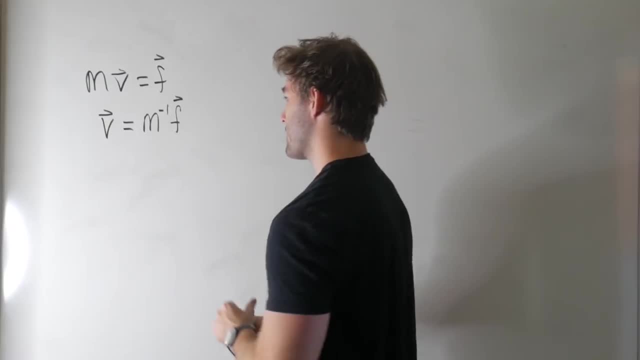 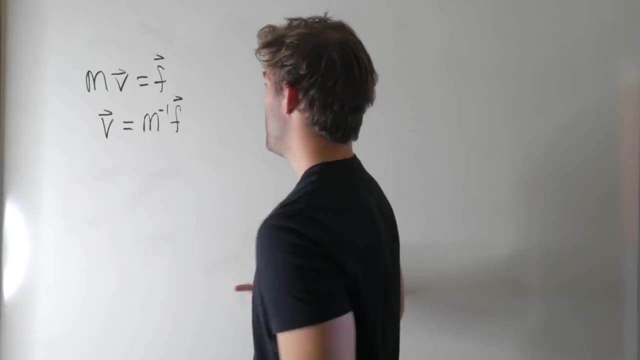 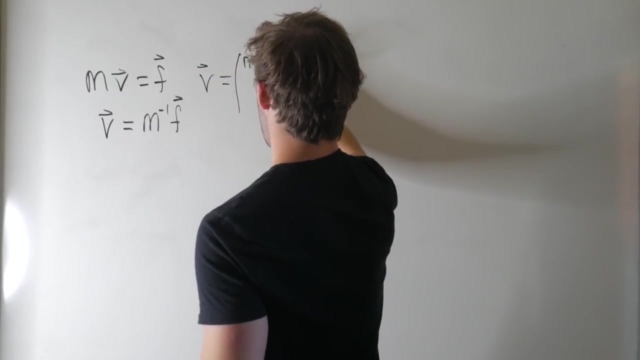 just to really be able to paint a picture of some important aspects of this. So let's say that M is a 2x2 matrix and the column vectors both just have two entries. So in other words we have V, vector is equal to, let's call it, M11.. I'm going to make it a bar. 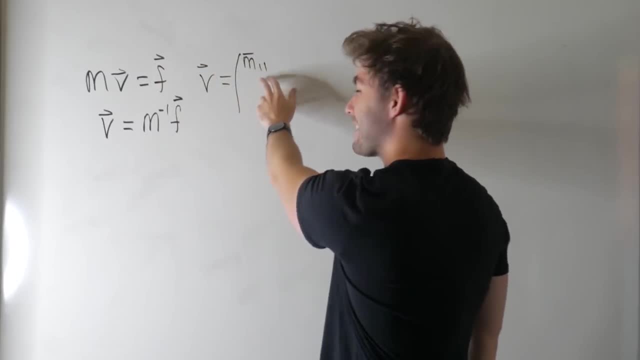 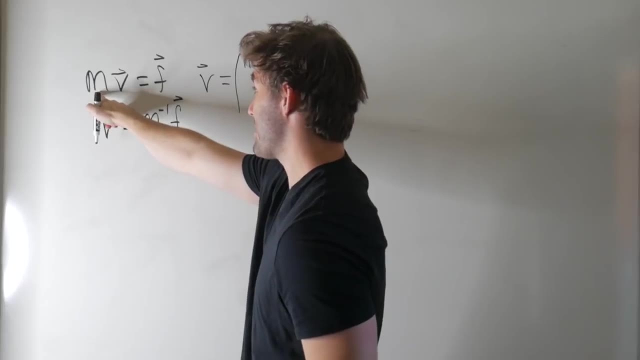 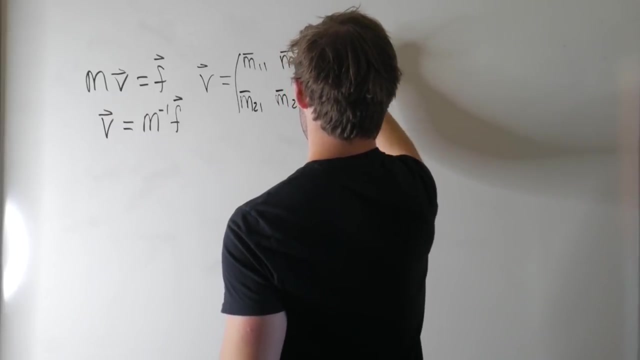 but this bar is not the same thing as these arrows, because I'm not saying that the matrix elements are vectors. M12 bar. I'm just trying to distinguish it from the matrix elements of M, M21 bar, M22 bar, times, F1, F2.. Multiply all this stuff out, so we've got. this is equal to. 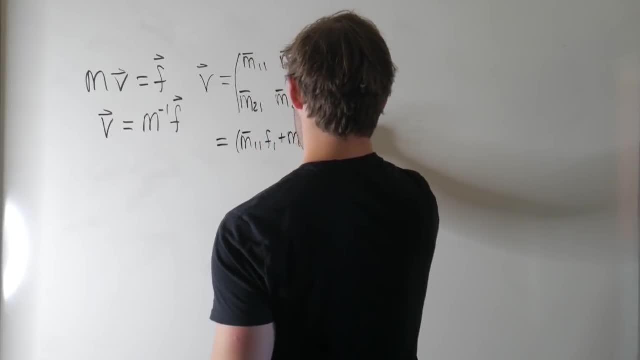 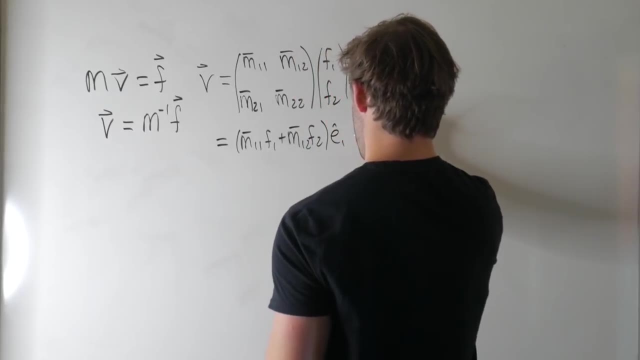 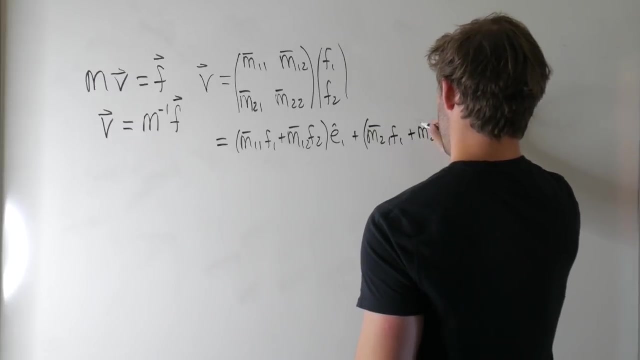 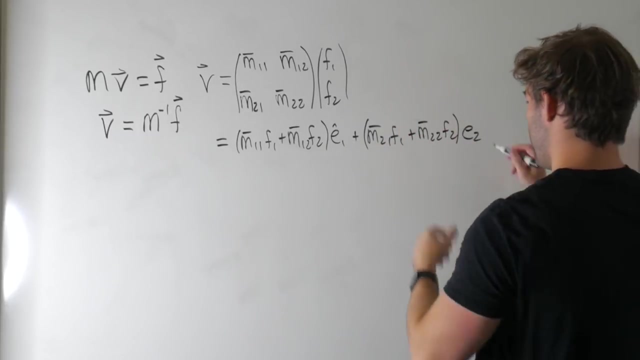 M11 bar F1, plus M12 bar F2.. And then this is going to be our first basis vector times our first basis vector, plus M21 bar F1, plus M22 bar F2, times our second. So this could be our x hat or our i hat and our y hat, and so forth. 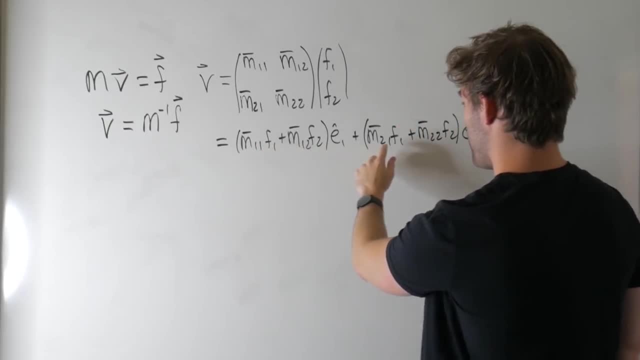 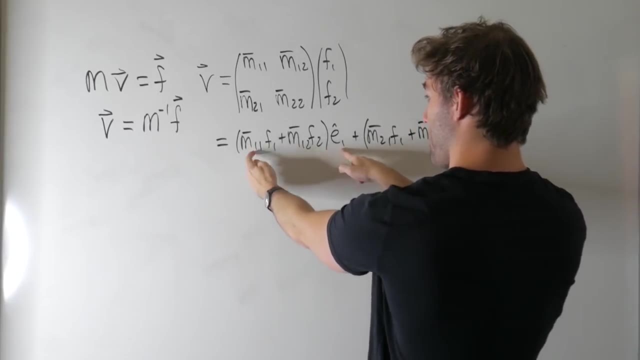 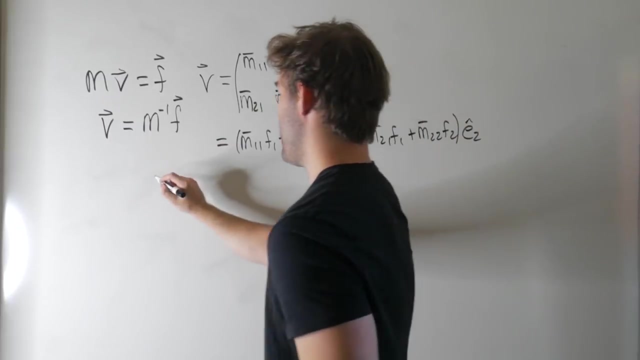 And we see a pattern here. The second index is being summed over 1,, 2.. And the component of the, so the x component, for example, is going to match the first index. So we can simplify this a bit. We can talk about a component of this vector Vi. 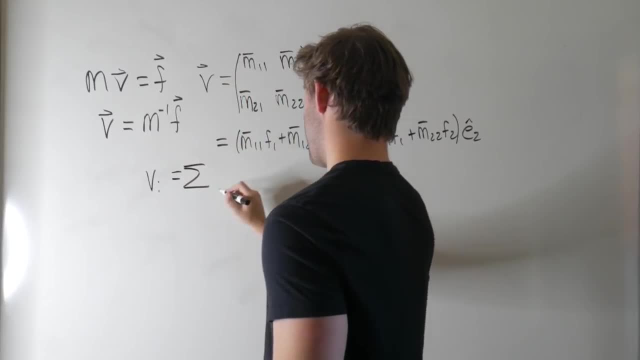 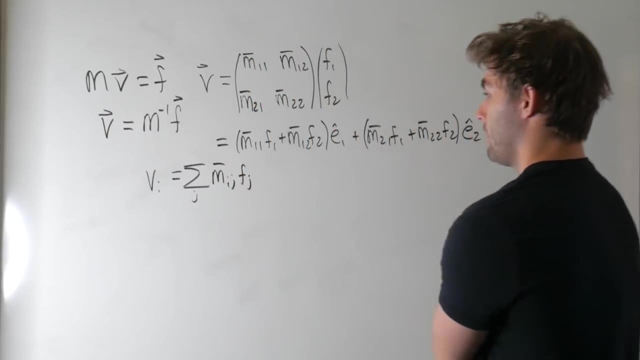 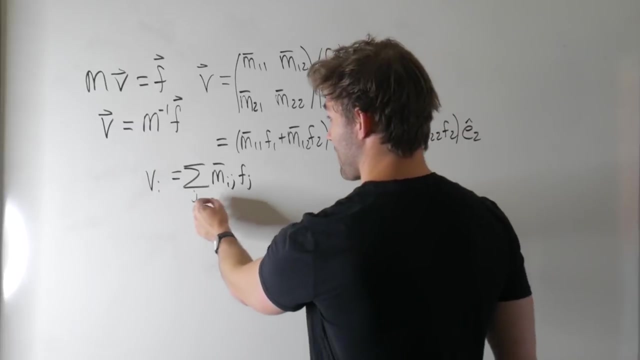 is just equal to a sum over some index, that second index, let's call it j- of Mij Fj, Cool. So what I'm trying to say here is we're characterizing a matrix by two indices, We're characterizing a component of a vector by summing over the second index. 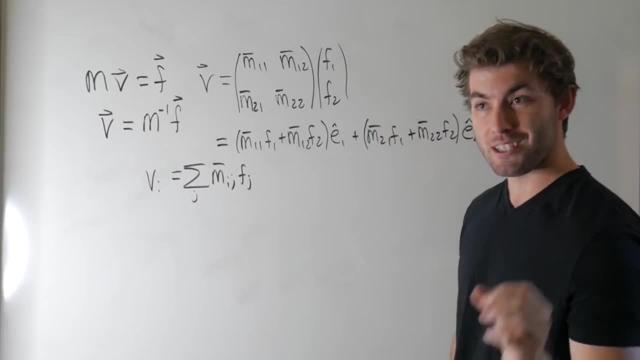 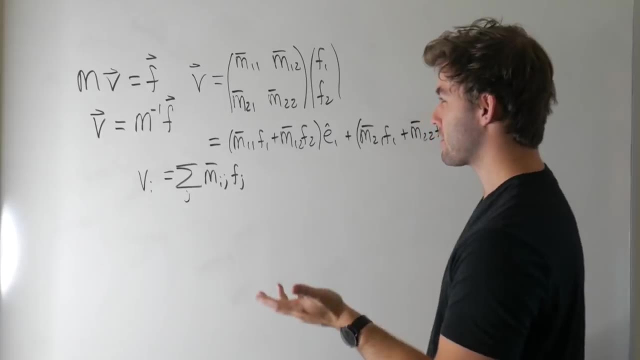 This might seem really abstract, and what does this have to do with Green's functions? but I'm about to get to it. Now I want to change gears and talk about something that's seemingly unrelated to this, but I promise it's not, And we're going to talk about differential 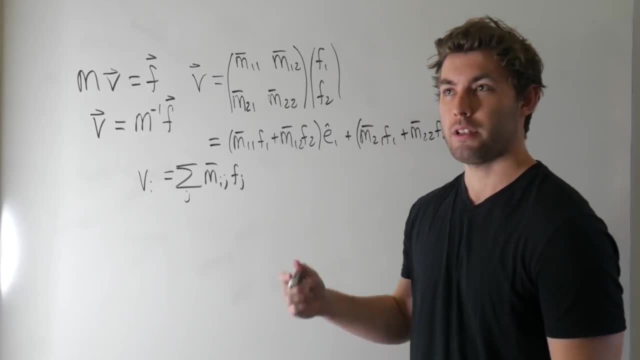 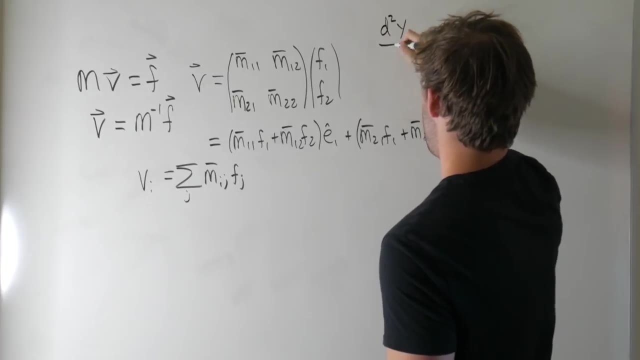 equations. So if we construct some arbitrary second order linear differential equation that looks maybe something like this, it doesn't have to look like this. it does have to be linear. d squared y, dx squared plus k squared y is equal to some function f of x. 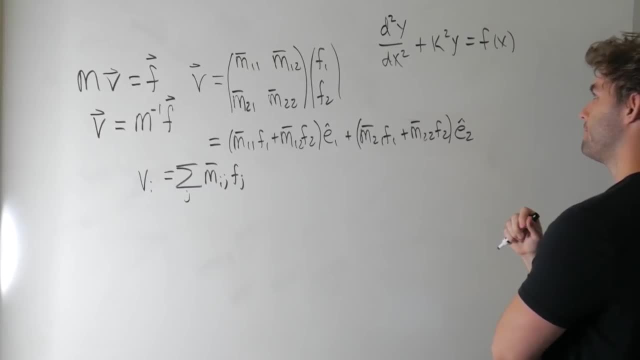 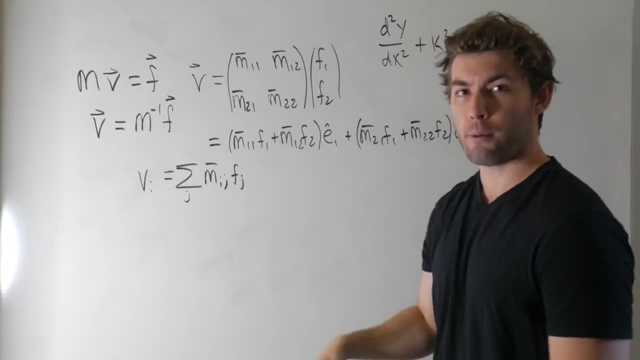 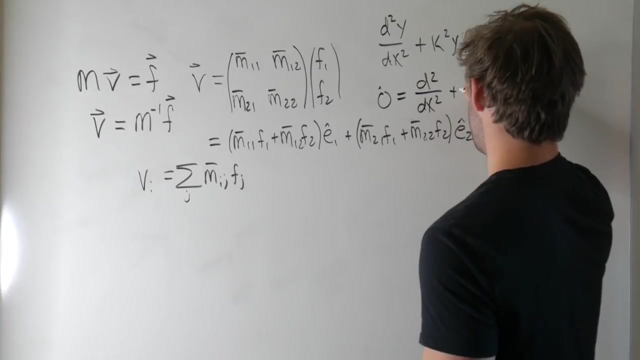 Okay, we're assuming y just has x dependence. Well, we can define some operator. If you've had quantum mechanics, you're familiar with defining differentials as operators. So we can define some o and define that equal to d squared, dx squared plus k squared, So o acting on y. 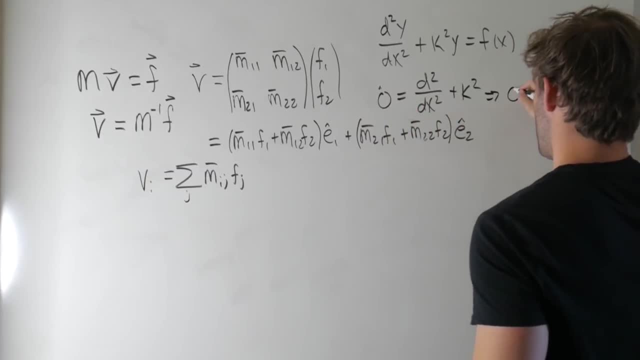 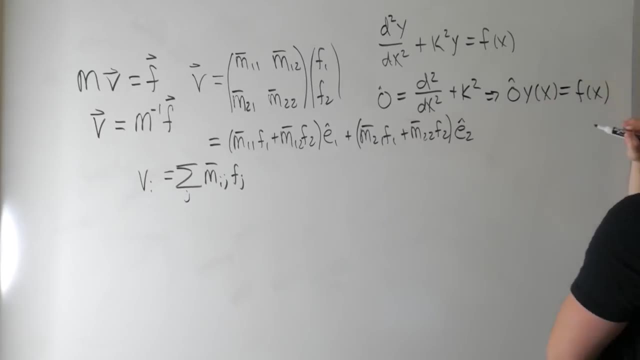 these just distribute, so to speak, and we get o, y. let's call it: y of x is equal to f of x, So this just reproduces this. This is just another way of representing this, But this looks an awful lot similar to this equation here. There we're dealing with vectors. 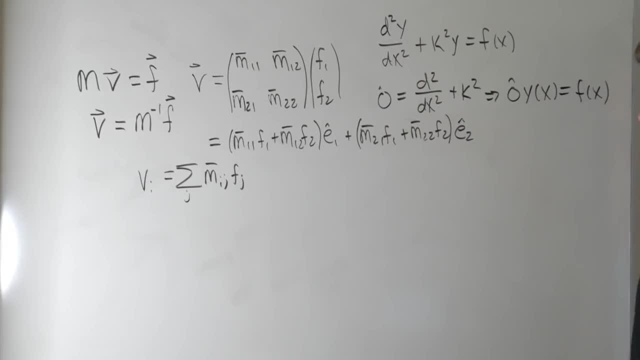 Yeah, here we're dealing with a scalar function, So it looks really more like this than anything, because this is just a component of the vector which would be a scalar. So then you're tempted to ask: well, what is the inverse of an operator? Can I say that y of x is equal to whatever this? 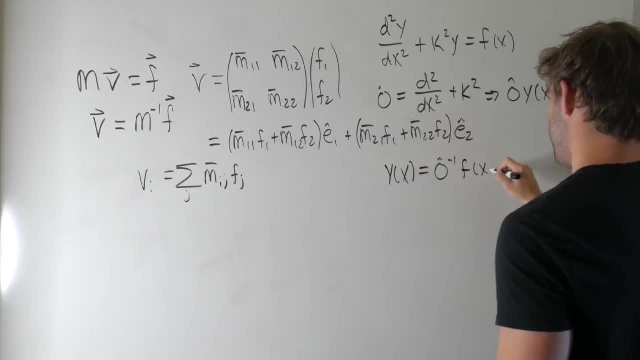 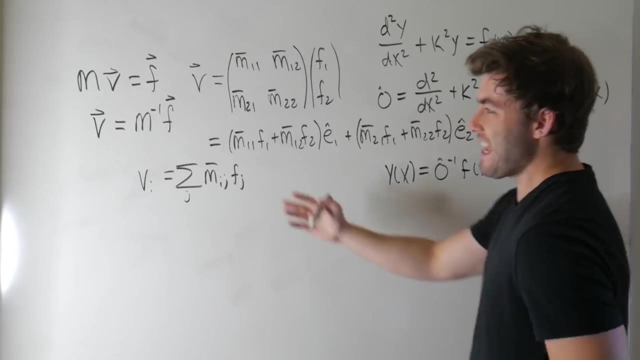 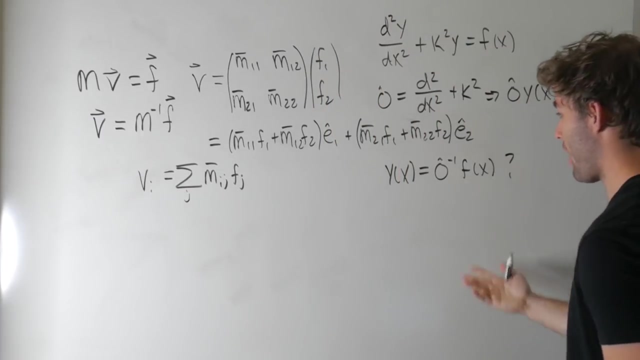 inverse operator is acting on f of x? And the answer is yeah, sometimes. Sometimes you can Just like how. sometimes you can't take the inverse of a matrix because it might not be invertible. sometimes you can't find the inverse of an operator. 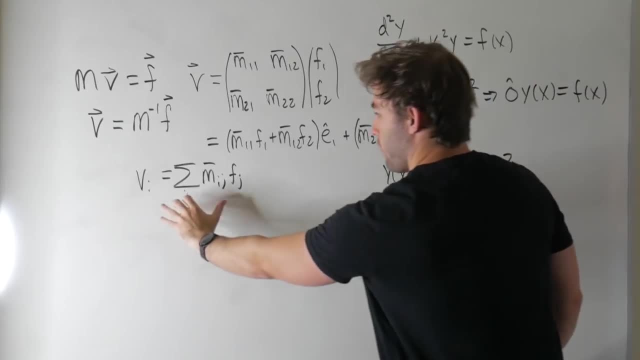 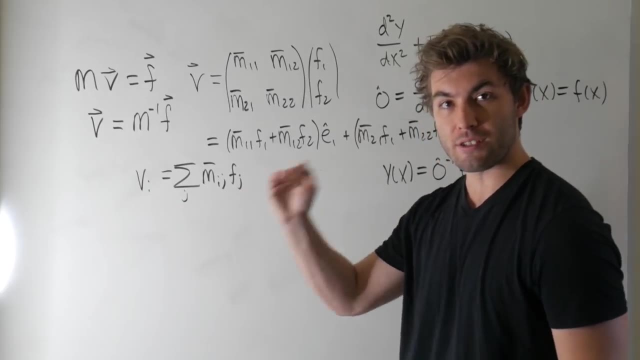 Now, when you look at this equation, this looks an awful lot like this one. The only difference is that the i is substituted for the x. The x is a continuous variable and the i is probably discrete. Well, also, this one has a j in it. This one has some other index and this doesn't seem to. 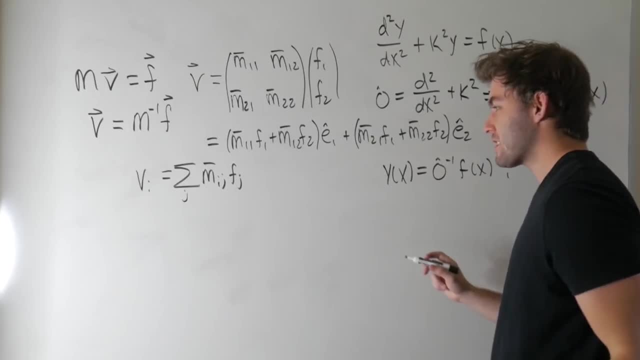 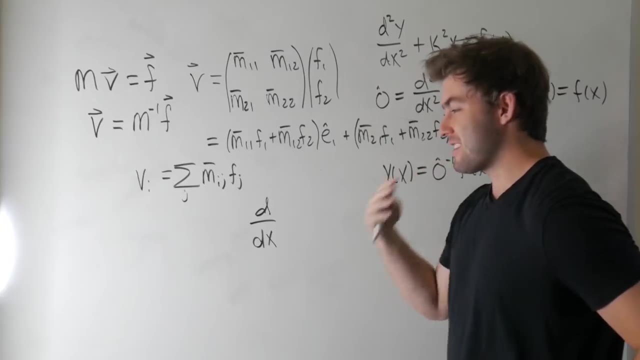 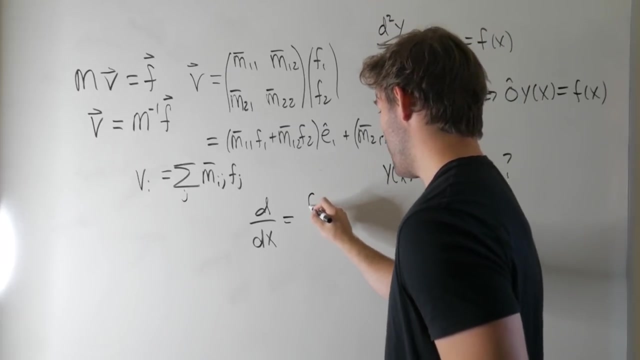 but it does. But it's hiding Whenever we say something like d over dx. this is an operator, but the second index that j has already been summed over, so we end up just writing this: But this is really in continuous space. 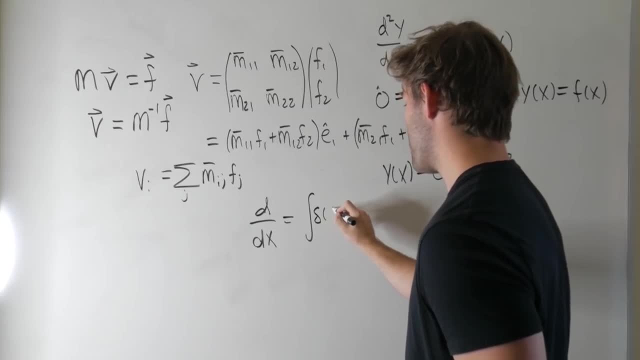 this sum becomes an integral and we get an integral of a delta function where we get some x minus x, prime, d, dx, prime. and let's have this act on some function. Let's call it q, Why not, just to be thorough? 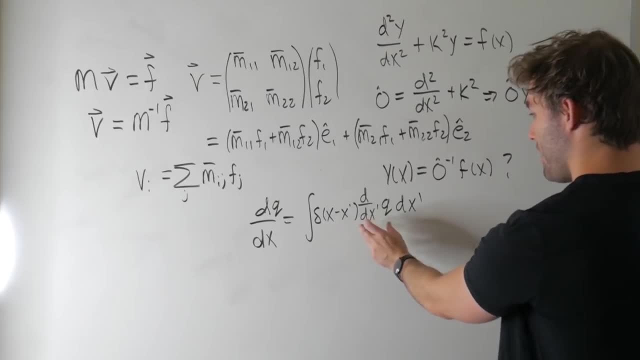 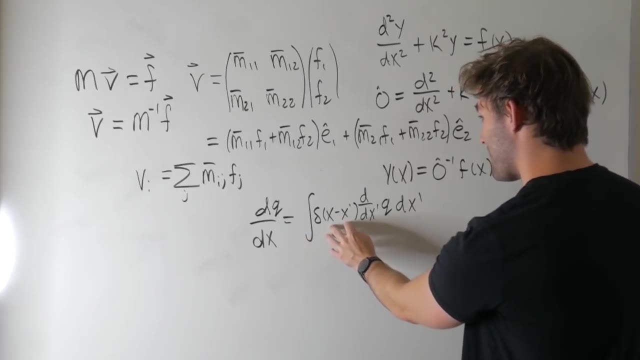 So this is picking out the value for x equal to x prime, and then we end up just getting the derivative of q with respect to x. So this is the real operator that has two indices, where that second index is summed over and in continuous space that sum becomes an integral. 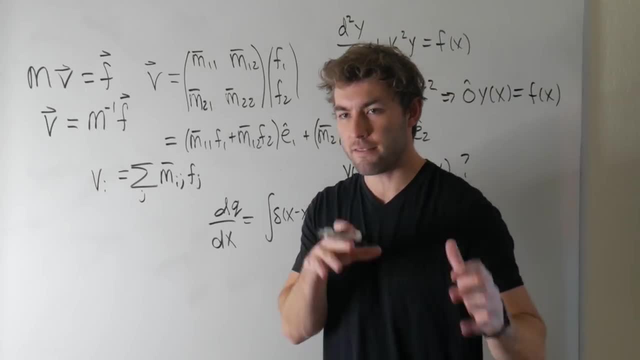 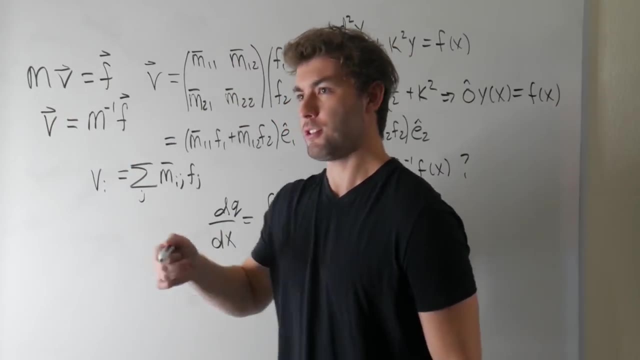 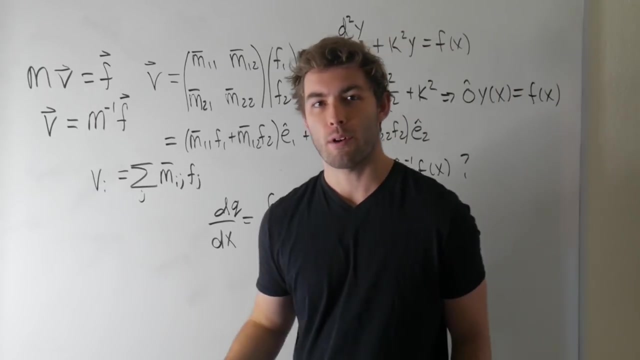 So when considering these inverses we're considering the inverses of some differential operators. So here, when we have a matrix acting on something, we can undo that act. by multiplying that by the inverse right, We get the vector back. So if we have some differential operator, 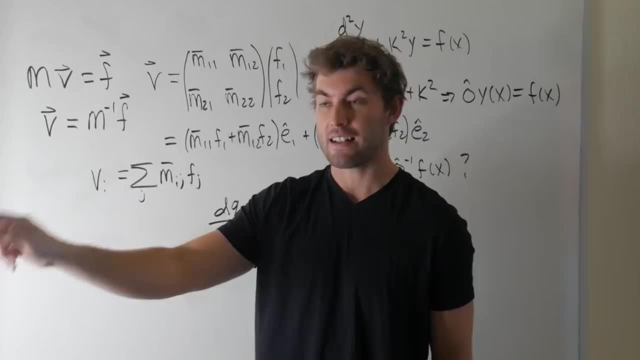 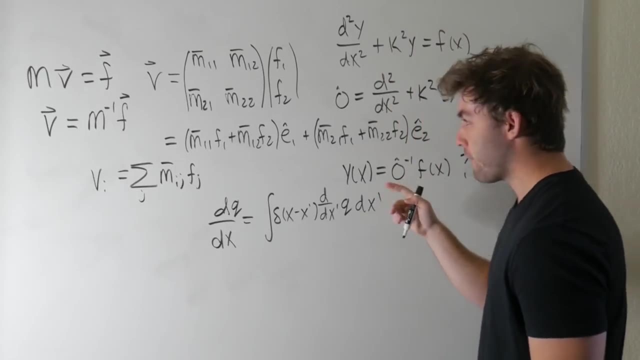 if we take the derivative of something, it would make sense that we get back that something by taking the integral right. The integral of the derivative gives you back the function. Uh, so it makes sense that the inverse of a differential operator would be some kind of. 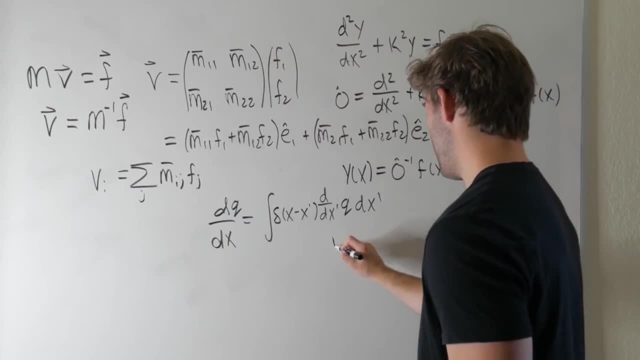 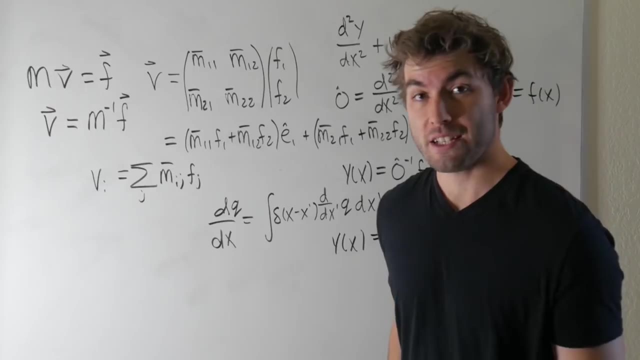 integral operator. In other words we got: y of x is equal to some kind of integral where we say the kernel of that integral is the Green's function, And so we'll call that, just like here, how we had some i and j. the Green's function should also have two indices, two continuous. 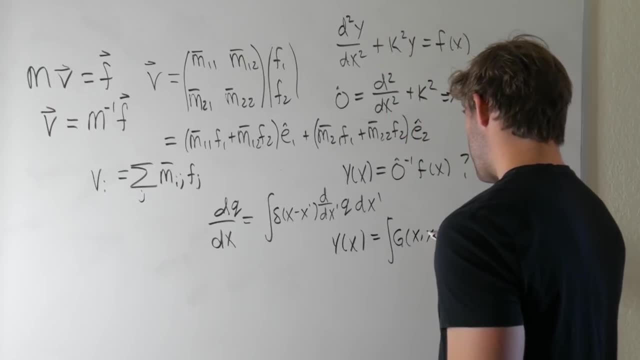 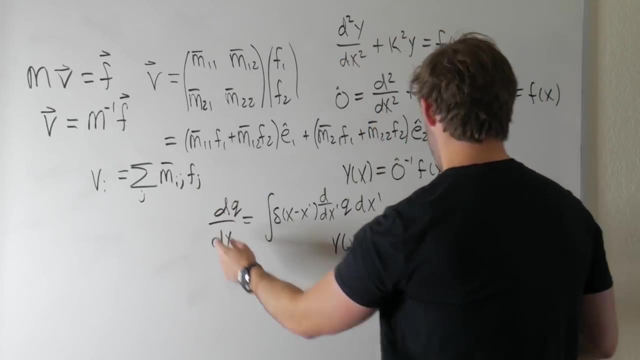 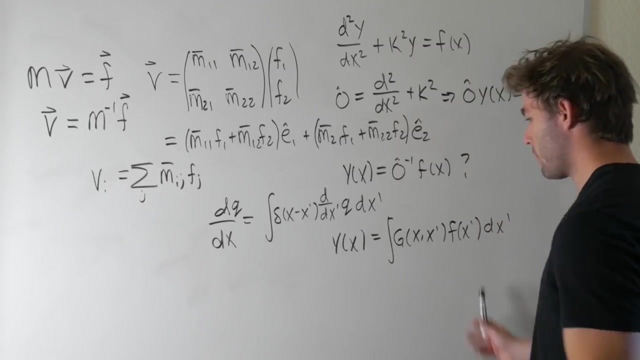 indices that we will call x and the z do x prime times. f. Here we have f of j, not f of i. Here we have f of x prime and we're integrating with respect to x prime. So what this whole thing tells you is that if you 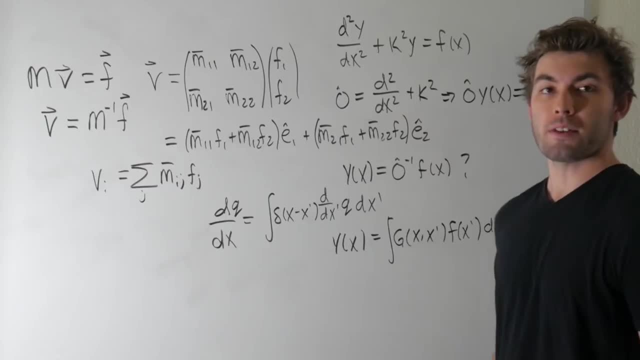 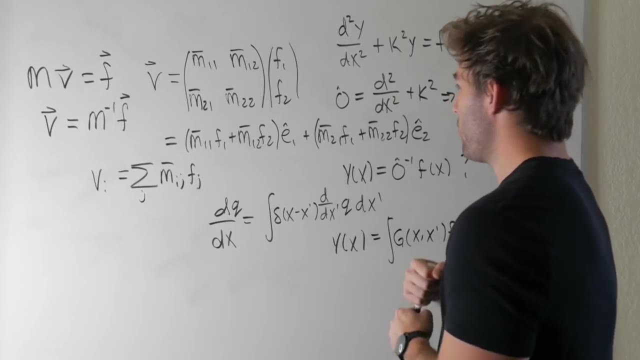 found the Green's function of the operator, you've solved the differential equation. But then the next question is: how do you find the Green's function? Well, in order to talk about that, let me erase this section here, just to make myself some room. Let's think. 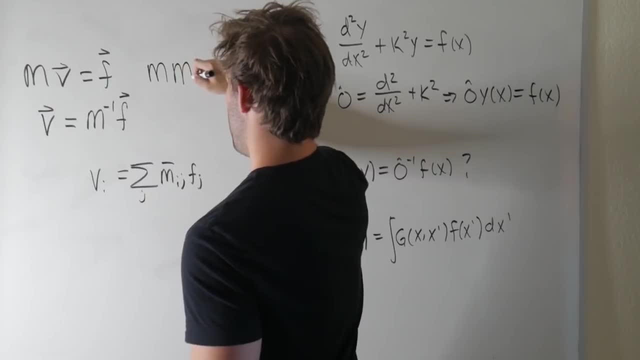 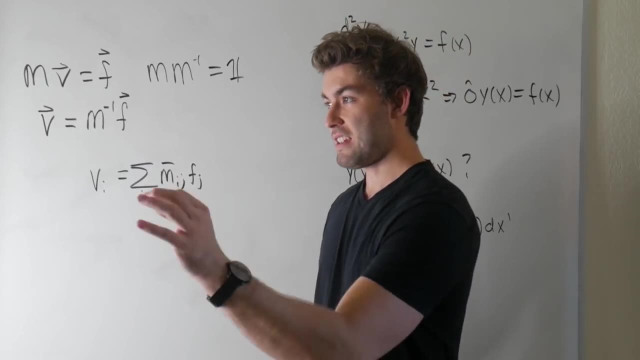 about what it means. if you were to multiply m times m inverse, That should clearly give you the identity matrix right, Also known as the Kronecker delta. If the index of the row equals the index of the column, you should get a one, or else you should get a zero Diagonals.